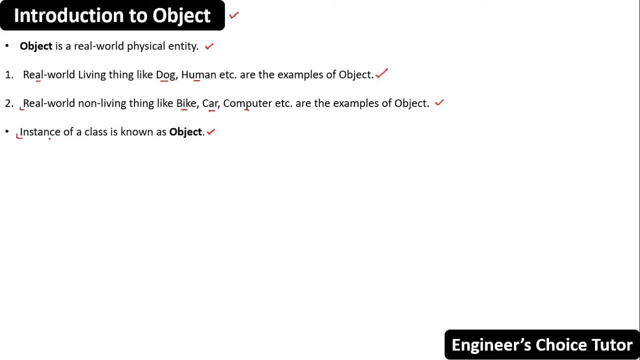 Now, you might be thinking, what do you mean? By instance. So basically, instance is nothing but allocating the suitable memory space for data members and methods. You know, there is one phrase. The phrase is instantiating a class. It means the same thing as creating an object of a class. OK. So using one class, programmer can create any number of objects. 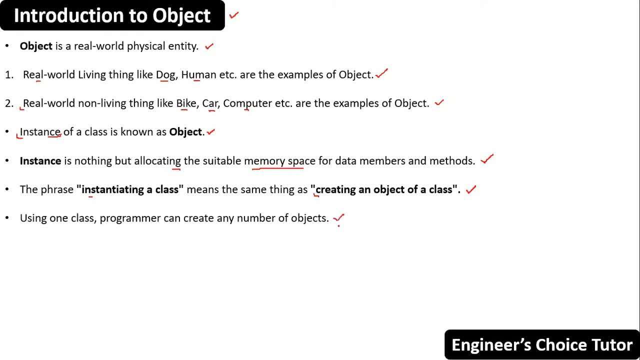 Remember this point. Fine. And every object has three properties. What are the three properties? First is the state. The another one is behavior. And the another one is what? Identity. Clear 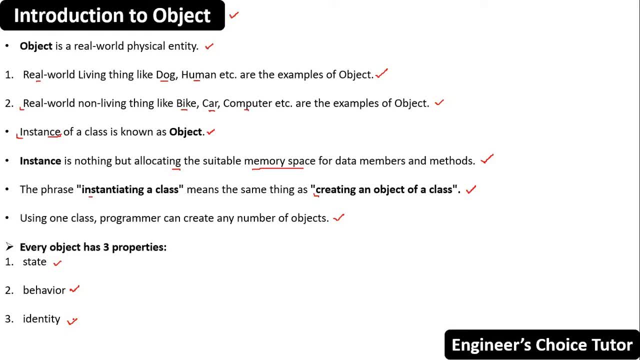 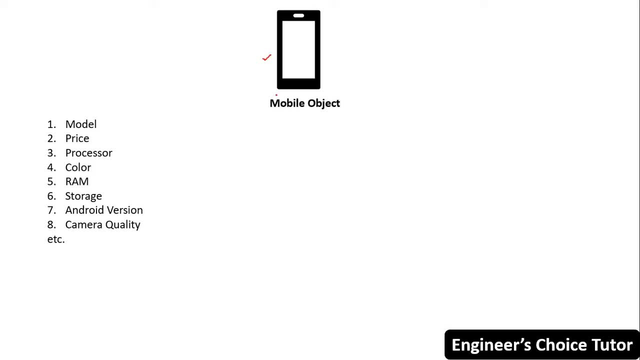 with this point? Now, let's understand the object with the help of example. So you all are using mobile, right? Mobile. So mobile is also what? A real world physical entity. So here we have mobile object. 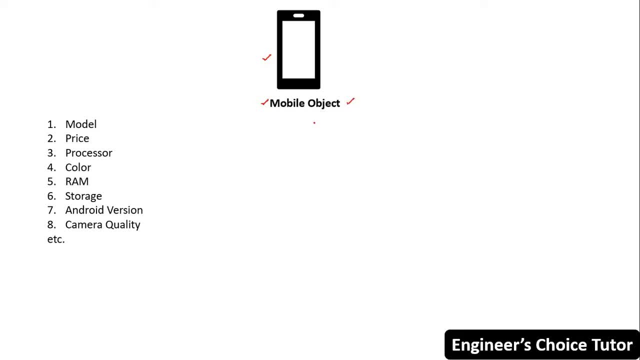 So you basically, state is its properties. Means state of a mobile object is its properties. For example, model, price, processor, color, RAM, storage, Android, camera quality, etc. All these things are what? The properties of the mobile. And this is what the state. A mobile object is the state of mobile object. So this type of object will be the mobile object. 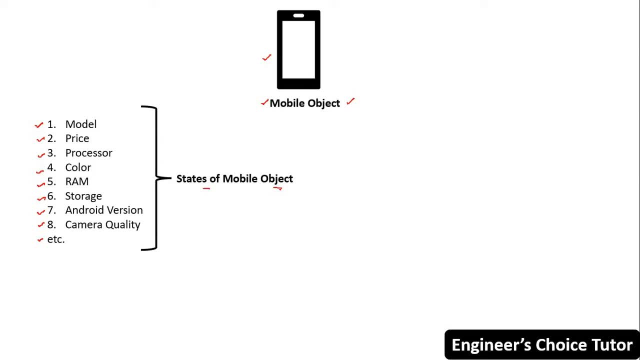 while object clear with this now coming to the behavior so basically you know what functionalities 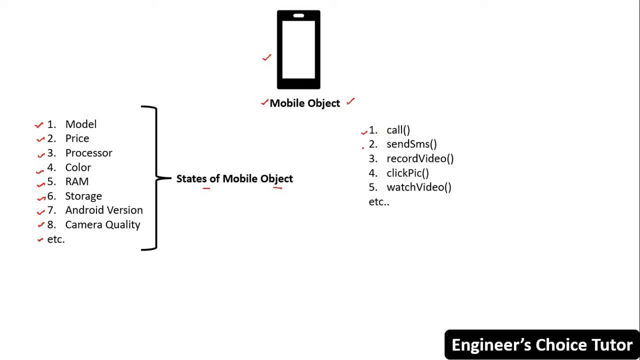 this phone can perform we can call by using this phone we can send sms we can record video we can click pick we can watch video etc many more functionalities right so basically behavior of 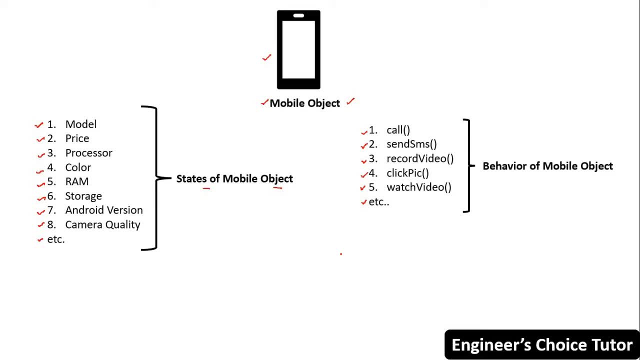 an object represents action or work performed by object clear so what do we mean by behavior and operation performed by an object is called behavior and coming to the states the value given 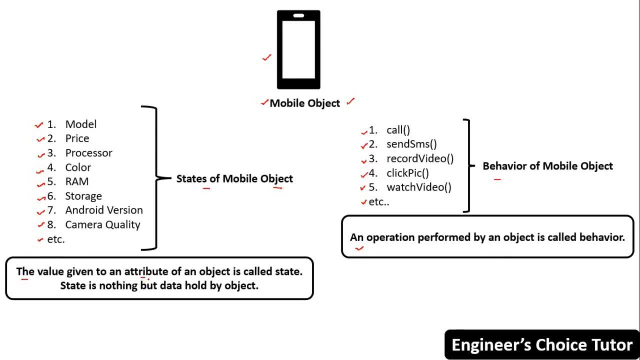 to an attribute of an object or property of an object is called state state is nothing but data hold by object we will see you 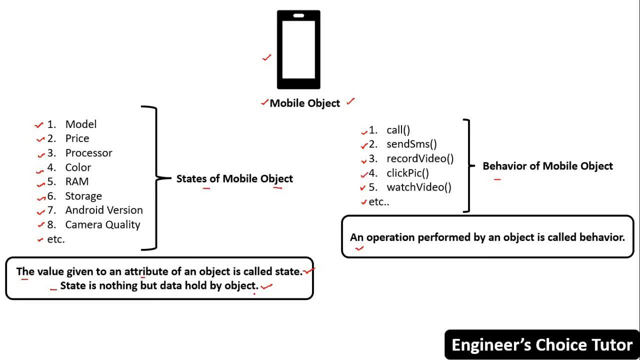 don't worry we will see how we can change the state using the behavior okay now the next 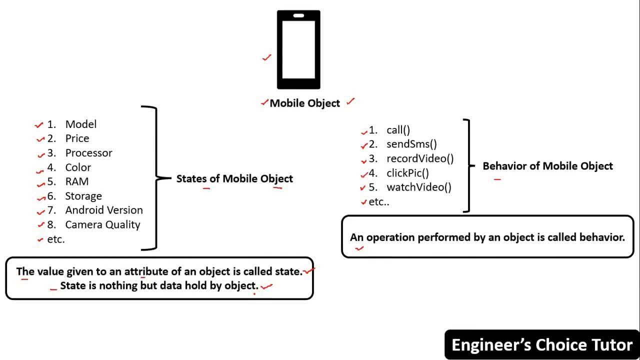 property is what identity right so basically coming to the identity identity is the hash code of an object it is basically used to differentiate one object from another object okay fine with this 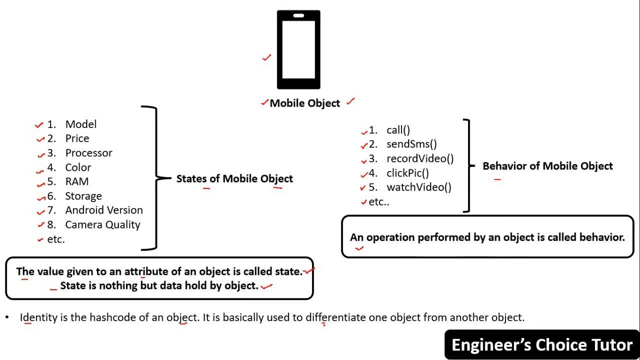 point so don't worry for now what is hash code we have to learn this thing in future for now just remember this thing that identity is the hash code of an object and basically used to differentiate 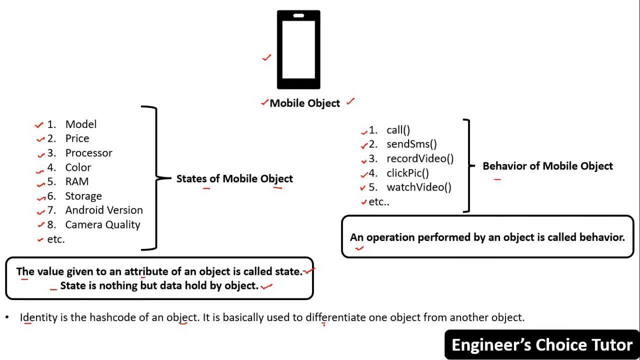 one object from another object so as we know and construction engineers takes the reference of 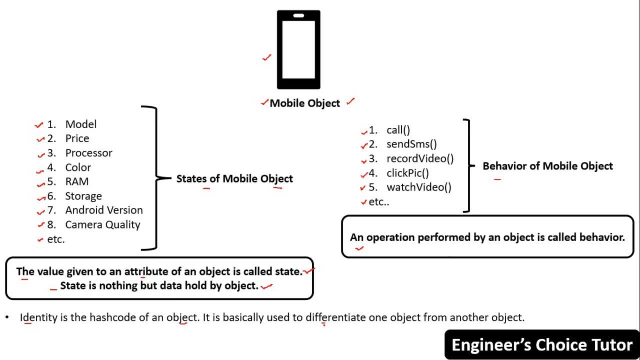 blueprint of home and then construct the home similarly jvm looks at the class which is basically what a blueprint of object right and then the jvm will create a object of that class 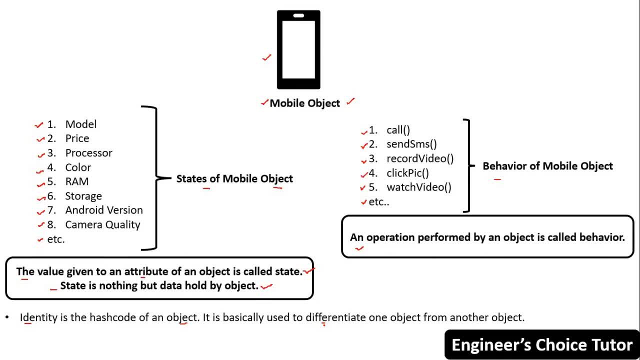 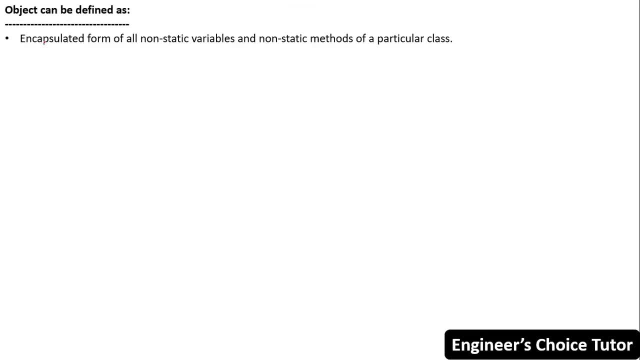 it will take the reference of what class to create an object remember this point so basically you can define object as encapsulated form of non-static variable and non-static methods of a particular class is called as object now you are not knowing anything about what is non-static and what is 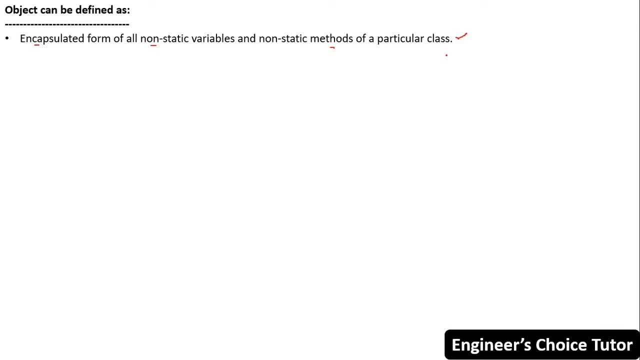 static right you are not knowing this thing so don't worry we will learn non-static variables and non-static methods of a particular class and we will learn about non-static variables and non-static variables static methods in the further lecture so this point is clear to you okay for now just remember 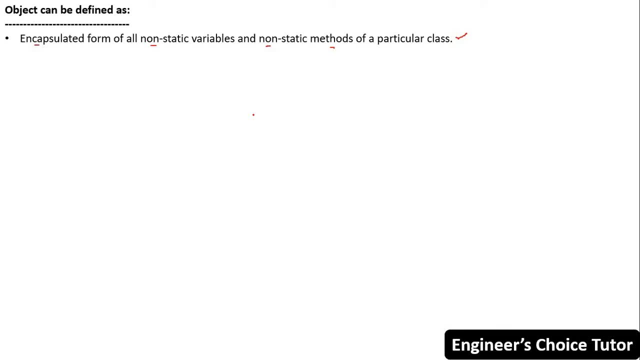 this definition so before going ahead after that what we have to see okay i understood what is the meaning of object but in java how can i create a object of a class so you know before going ahead 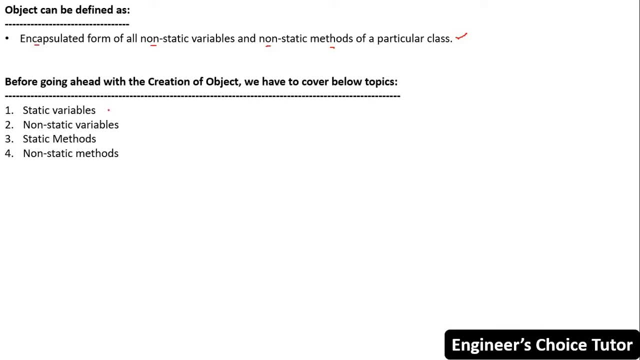 with the creation of object we have to cover below topics what are that topics static variables non-static variables static methods and non-static methods so after completing these topics we will see how to create an object in java once you are done with this you know it is very easy for you